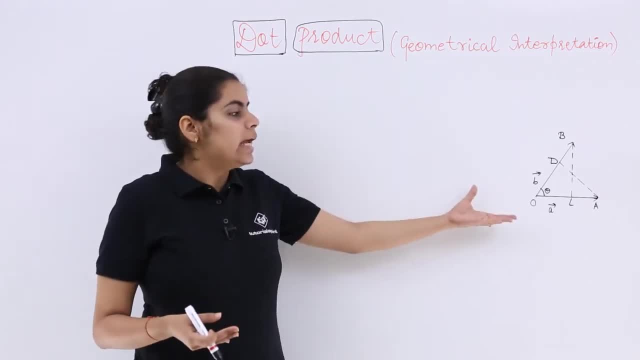 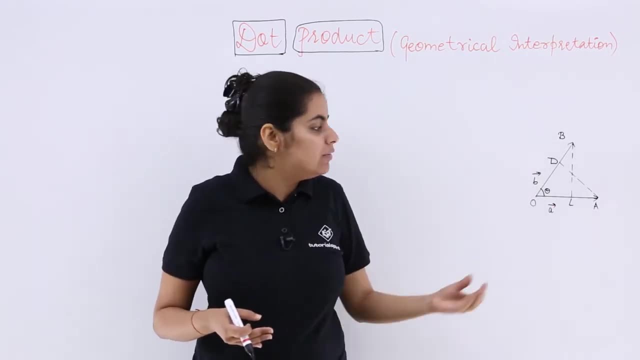 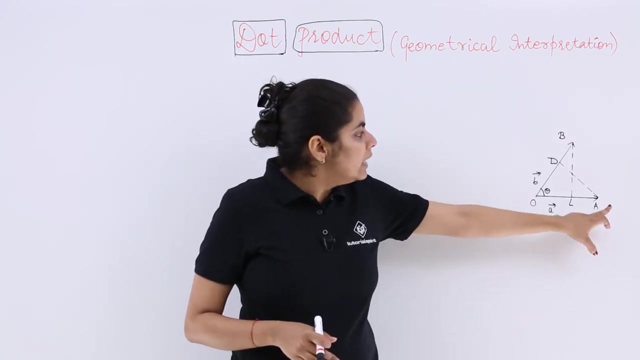 Let's see what is the geometrical interpretation in case of dot product. So I have this diagram. Let's see. these are the vectors, OA and OB respectively, which can be named as A vector and B vector. Let us draw a perpendicular: BL on OA and AD on OB. So these are the perpendiculars. 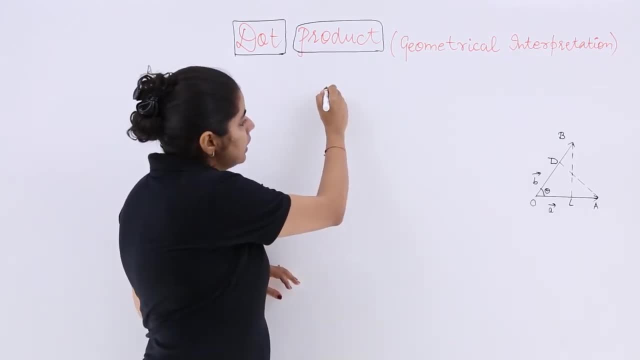 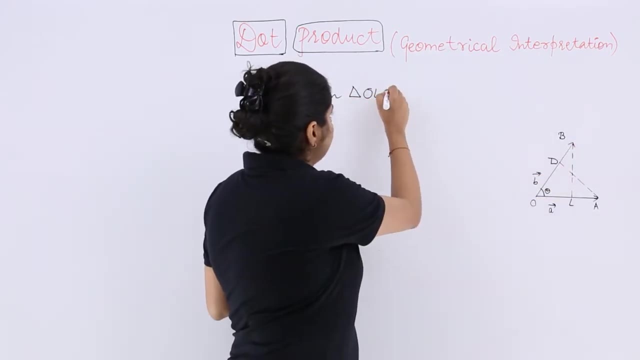 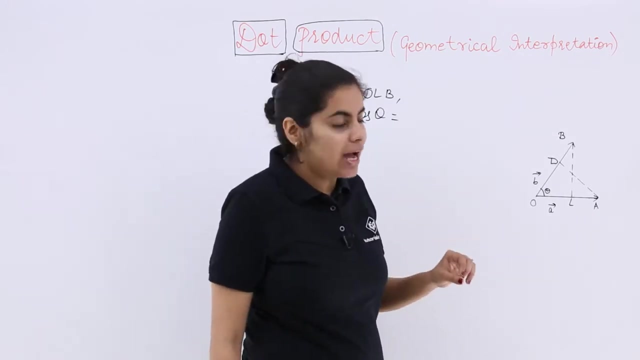 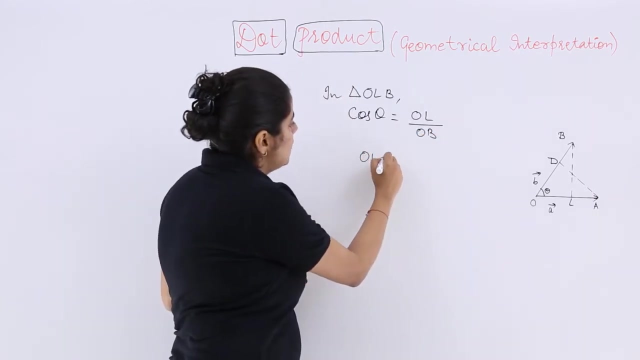 Now just let me know one thing: What is the in triangle, in this right angle triangle, OLB? what is cos theta? So cos theta is base upon hypotenuse. So what is base OL upon hypotenuse is OB. So I say that OL is equal to OB, cos theta where OB is what. 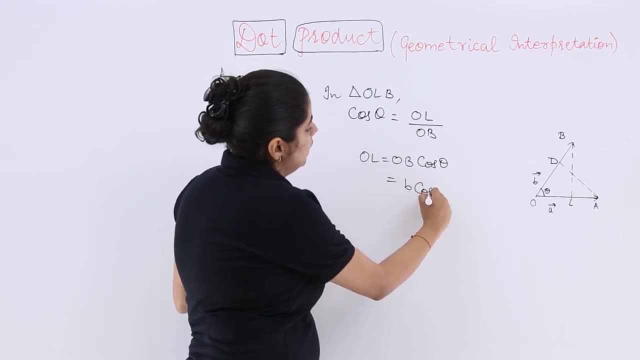 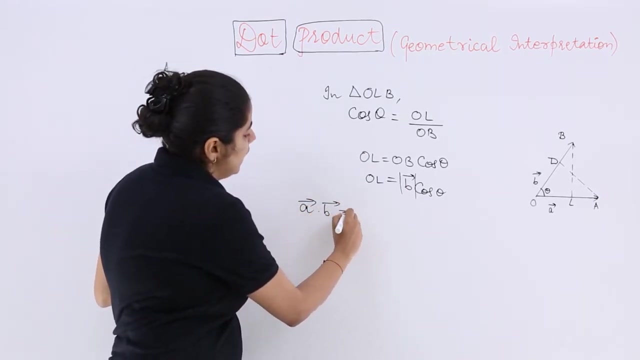 Where OB is equal to OB cos theta. So I say that OL is equal to OB cos theta. Where OB is B, So it is B cos theta. This is OL. Now this can also be read as magnitude of B cos theta. Now, this is done. Now you tell me what is the dot product of A and B. 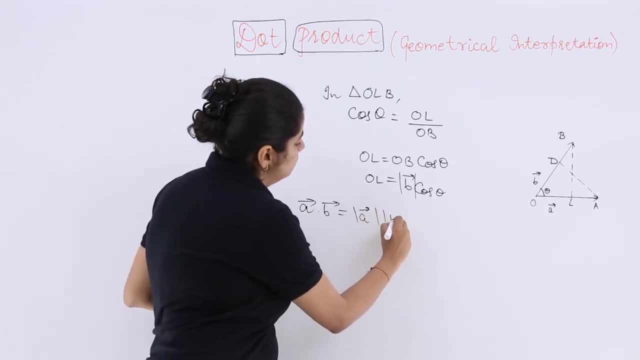 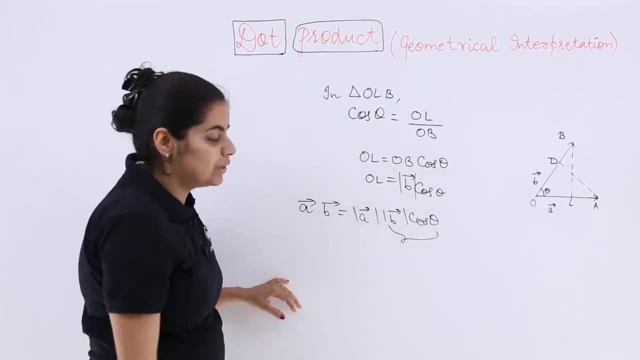 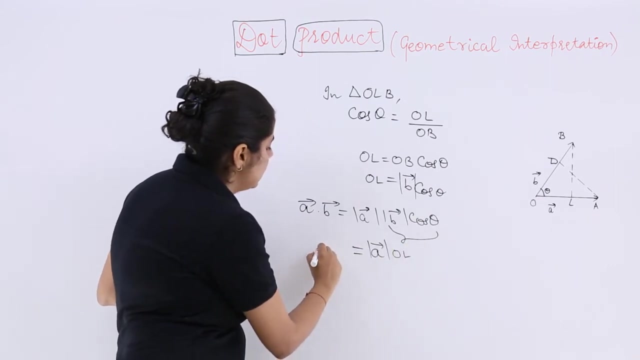 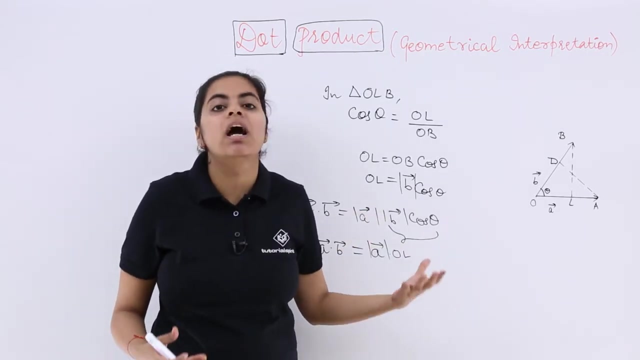 vectors. It is AB cos theta And simply this B cos theta can be substituted as OL. So it is A multiplied by OL and that is A dot B vector. Now see, in terms of projection, how can I say the dot product to be like. So the dot product of A and B vector is actually equal to the 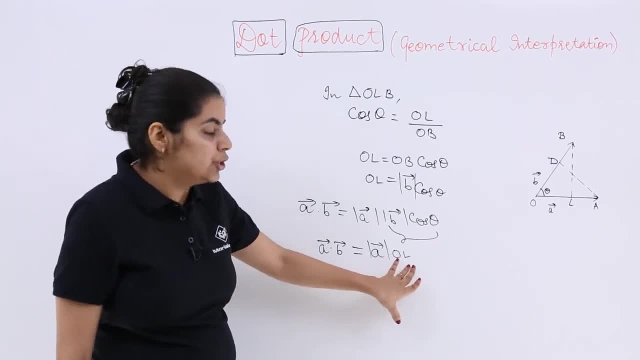 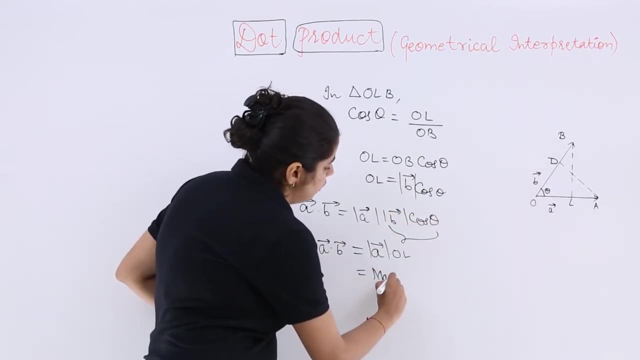 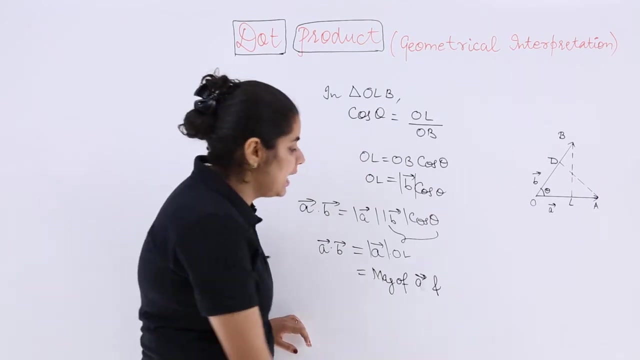 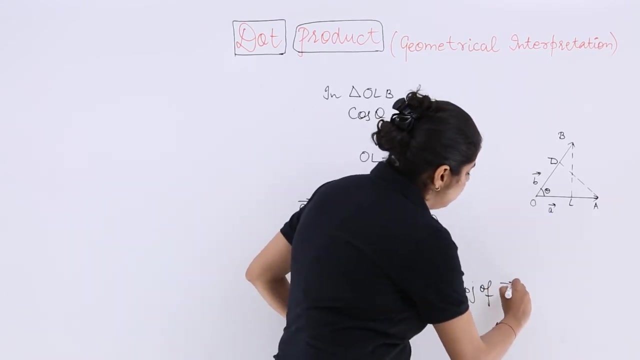 dot product of the magnitude and the projection. The projection is OL, which is the projection of vector B on A. So I say magnitude of A. So this is the dot product of A and B vector. So the dot product of A and the projection of B vector on A vector. That is about the 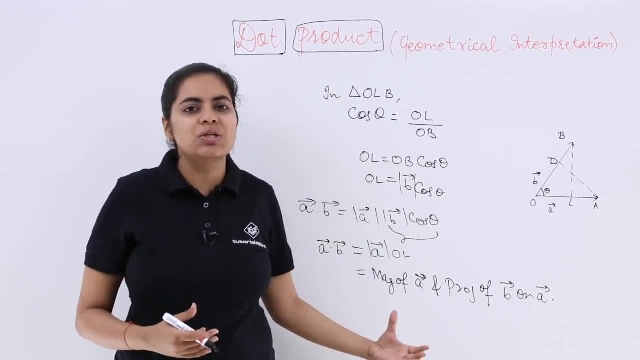 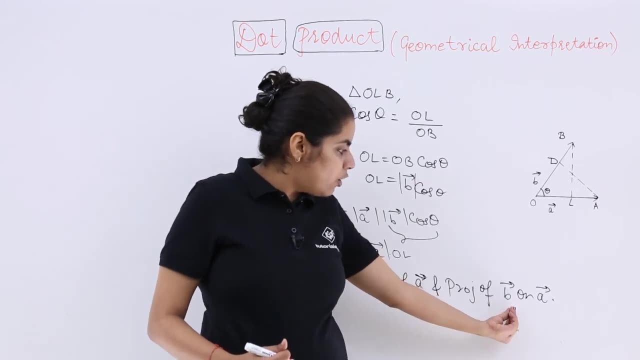 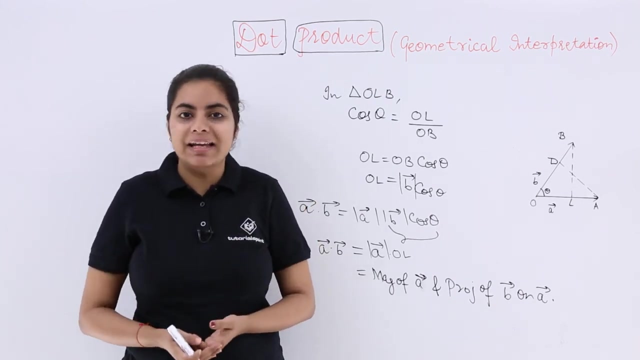 dot product. Similarly to this. as you did this, you can write the A dot B as magnitude of B multiplied by the projection of A on B. That is the homework for you. So projection and the geometrical interpretation are interrelated.